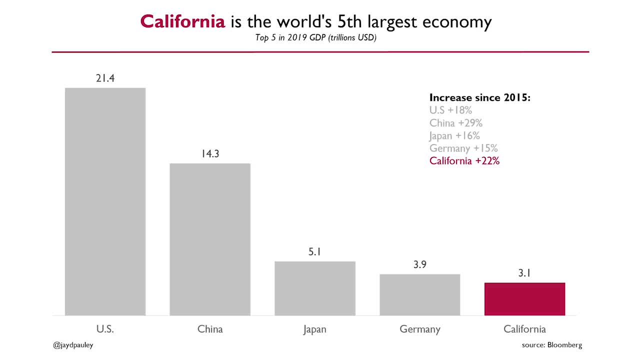 more than Japan, more than the United States overall and almost as much as China- China, a developing nation that is experiencing a rapid economic growth, expanding middle class, et cetera. China has grown twenty nine percent since 2015.. 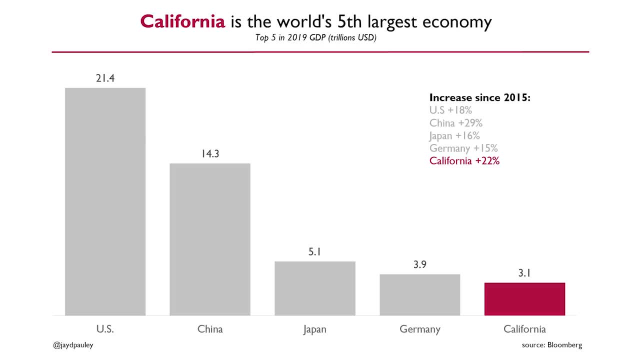 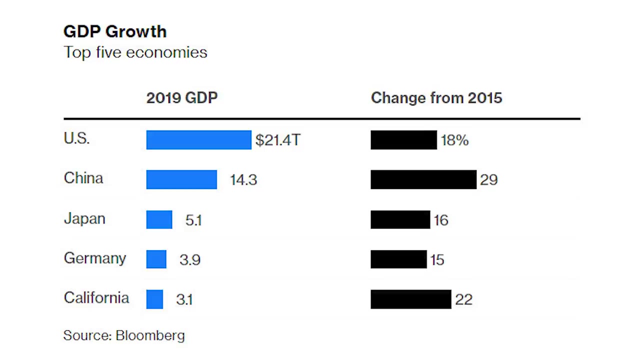 California has grown almost that amount, And in the midst of this they're trying to recall Democratic Governor Gavin Newsom. And yet the state is growing almost as quickly as China. California added one point three million people to its nonfarm payrolls since last April. Household income increased one hundred and sixty four billion dollars. 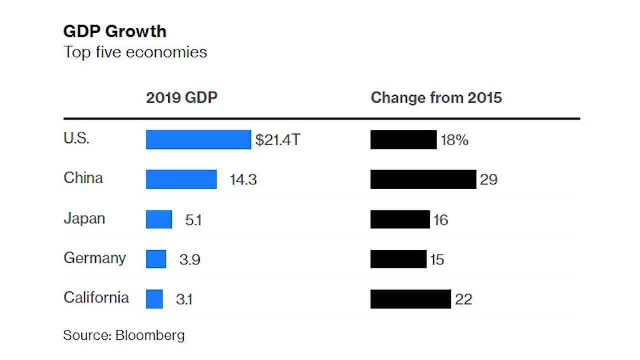 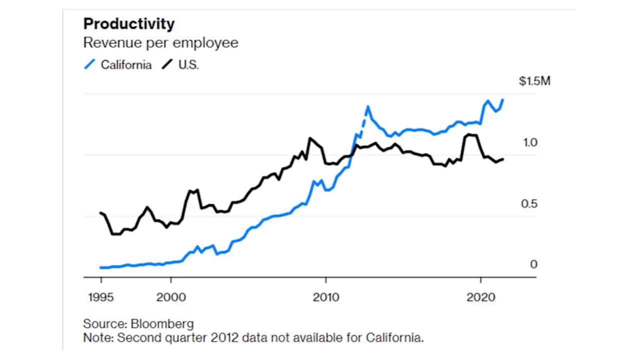 almost as much as Texas, Florida and Pennsylvania. California's budget surplus- Yeah, it's a surplus. You wouldn't know this from listening to Fox News about California. The California surplus has grown to a record seventy five billion dollars. Revenue per employee has grown in California much more quickly than in the rest. 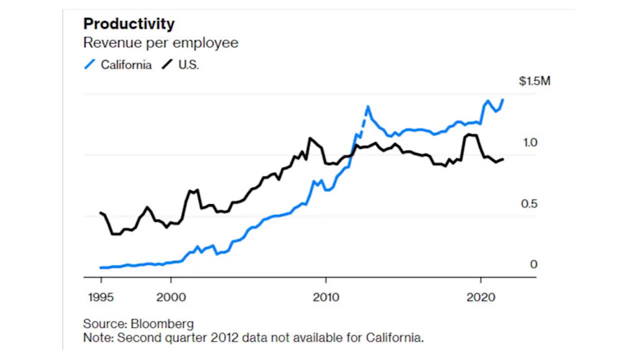 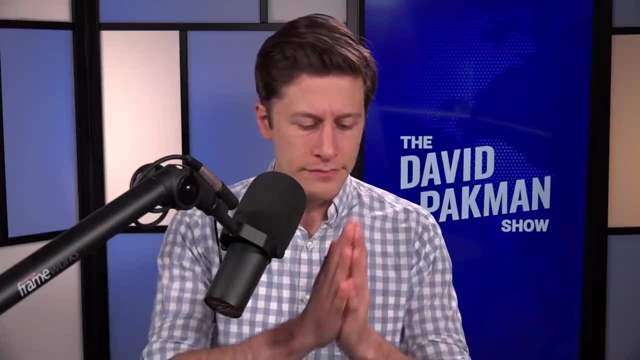 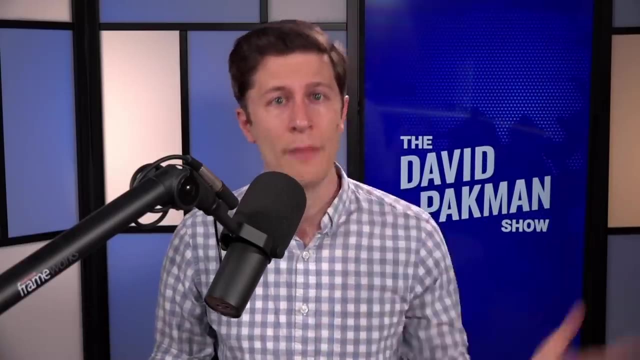 of the United States. So there are some really important takeaways here as we think about what the sensible economic policy look like At the state level. first of all, the constant, endless ranting from Republicans about how terrible everything is in California: economically, socially, culturally and otherwise. It's just not. true. Is California expensive? Absolutely, California is expensive in the net. Are taxes higher in California for someone of average income than in many other states? That really depends. There's this study that looked at Texas versus California. for someone making, I think it was like. $100,000 a year And if you really account for all of the expenses that are levied by the state in California versus Texas, And so you look at local and property sales taxes, fees on cars and other different things, It ends up being slightly cheaper to live in California. than Texas for the average person, even accounting for the California state income tax. But the more important takeaway is, you know more recently the covid lockdowns, as they were called, not that many people in California were even really abiding by the right, was saying covid. 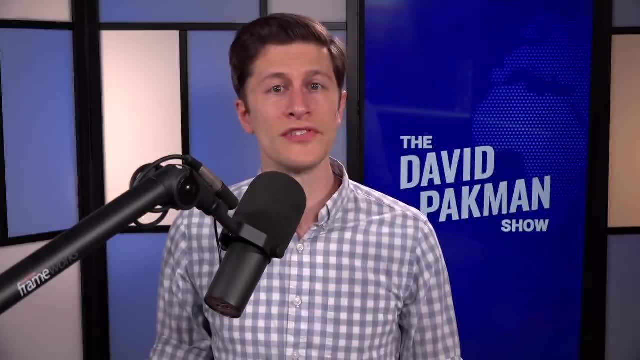 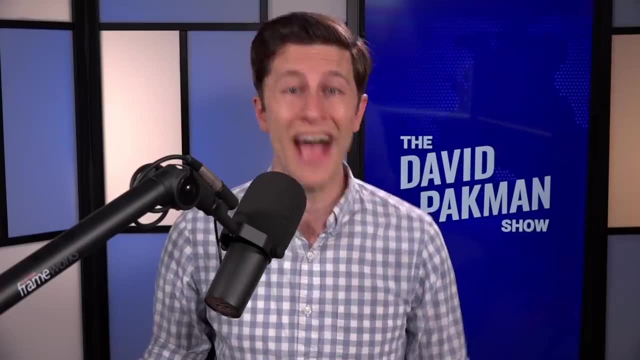 lockdowns are destroying California. They didn't destroy the state. California is doing really well. California is in the top states in terms of portion of its population vaccinated, which is sort of a logistical and infrastructure signal about California. So the bottom line is: 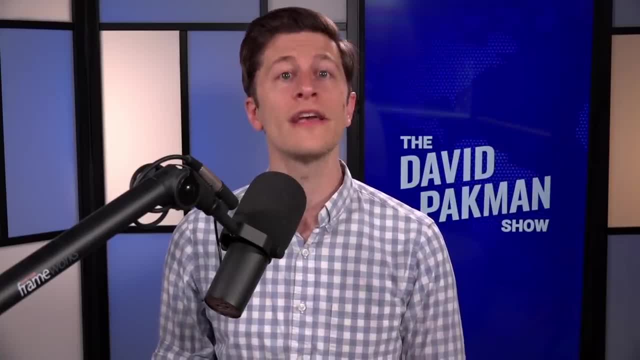 California is expensive, but it's expensive for a reason, And you would think that Republicans would understand this, The people who talk about the free market. the reason they're doing it is because they're doing it, because they're doing it for a reason. That California is expensive is. there's really high demand and a lot of people want to live there. Why do things cost a lot? Sometimes things cost a lot because lots of people want to buy them. That's called the market. Now, that being said, California, like every state, still has many. 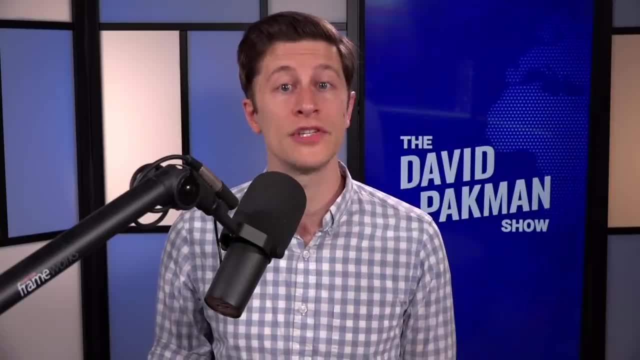 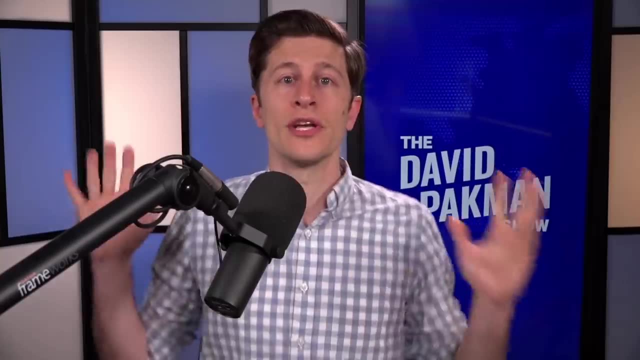 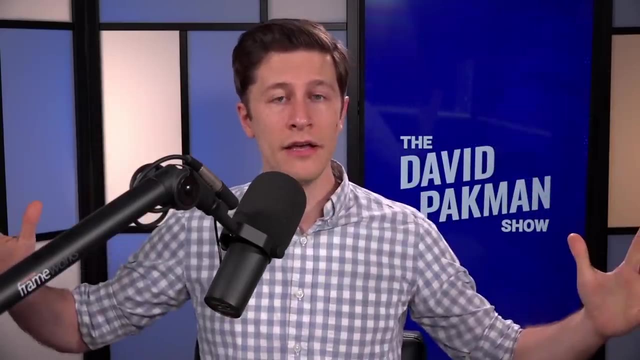 problems that many metro areas have. because it's in demand, It prices out lots of people, including people who want to live there but can't afford to. That's a real issue. We can recognize it's a expensive because people want to live there And that is a market based thing. But at the same time 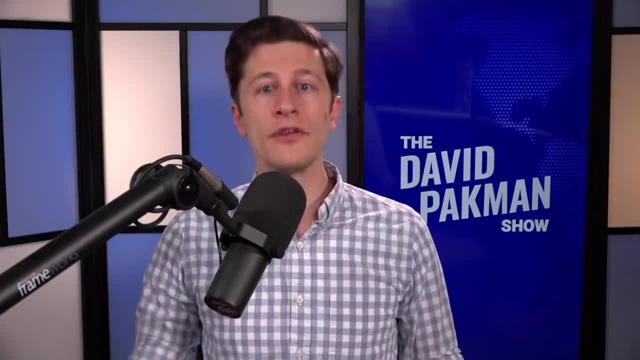 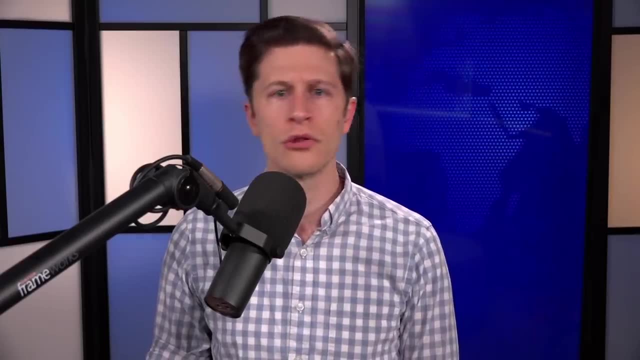 a lot of people are getting priced out. That's a real issue. We still have huge inequality in both wealth and income. California is no exception to that. But the lies that you're being fed by people like Tucker Carlson and Laura Ingraham and various of the Trump's and others about the dystopian 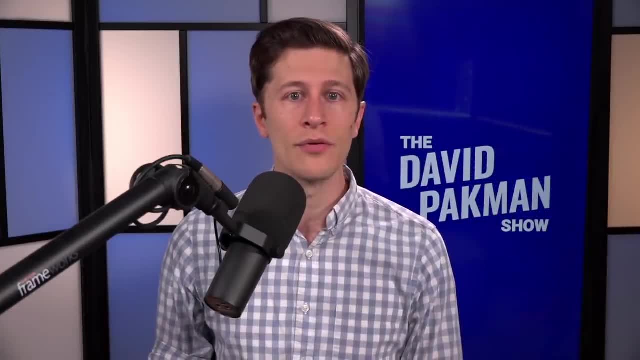 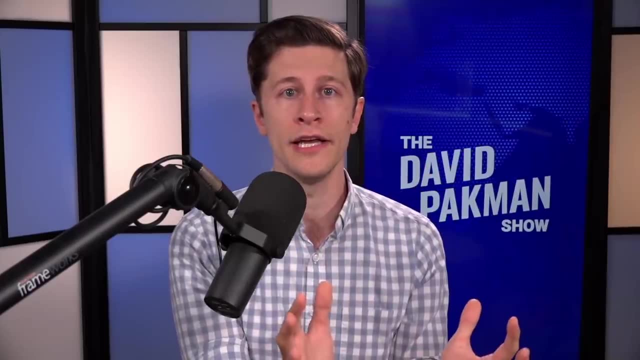 California. it's not true. The undeniable reality is that California is the envy of the world in terms of an economy. If California were a country, California would be the biggest economy in the country, It would be a significant country globally, and it's just one of 50 states in. 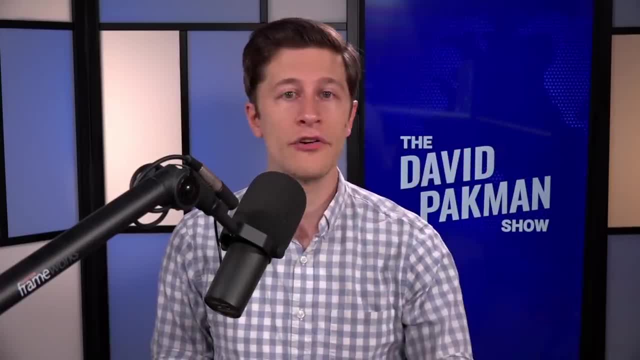 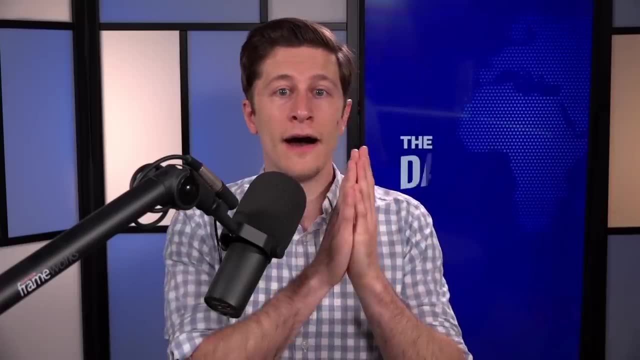 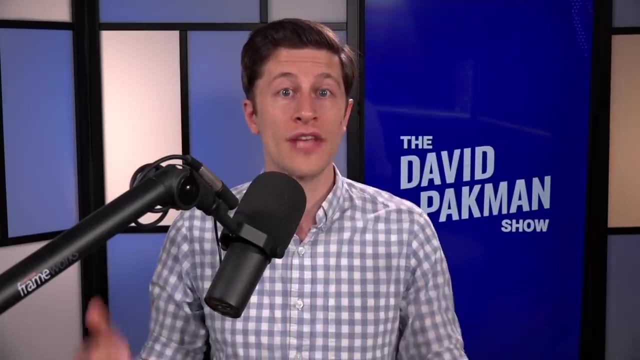 the United States in terms of average standard of living, in terms of innovation, in terms of technology. Some of the best places in the world to live are in California. They aren't in West Virginia, Right? I'm not attacking West Virginia or the people of West Virginia, But what I'm saying is: there's a massive infrastructure difference between California and West Virginia. There is a population quality difference, There's a massive health care quality difference, Wages are significantly higher, And yeah. so all of that together makes California expensive and it makes West Virginia really cheap. It has to do with politics, It has to do with demand And it's 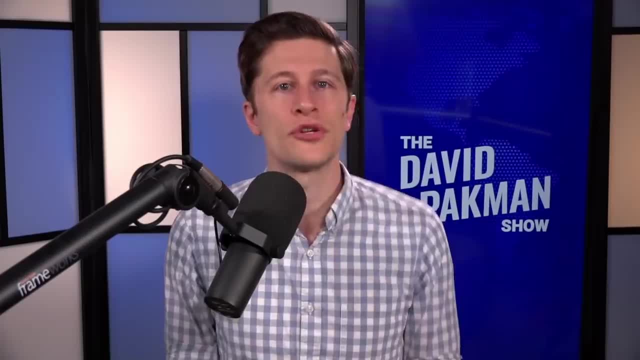 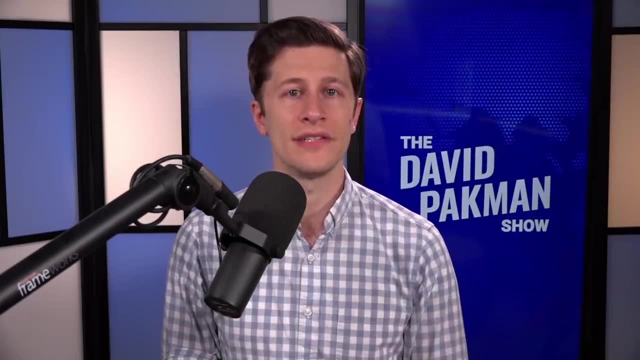 actually stunning that Republicans get away with trashing California when it's an obviously incredibly dynamic economy that, in many ways, is the envy of the world. California would be a globally successful country And it's an incredibly dynamic economy that, in many ways, is the envy of. the world. California would be a globally successful country And it's an incredibly dynamic economy that, in many ways, is the envy of the world. California would be a globally successful country And it's an incredibly dynamic economy that, in many ways, is the envy of the world. And 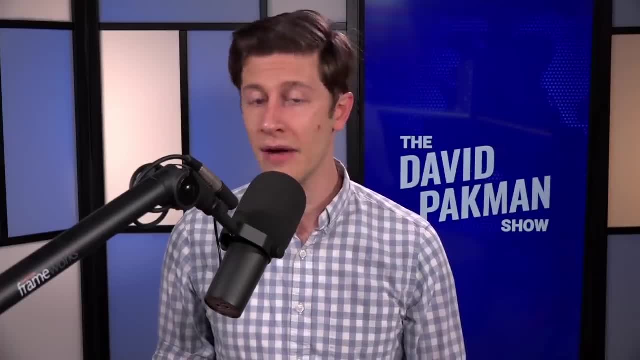 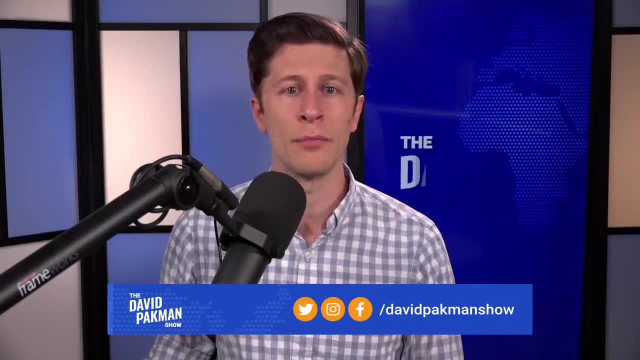 in the midst of this. are they going to recall the governor, Gavin Newsom? I don't know. We will see and we're going to follow it, But the doom and gloom about California, it is just not backed up by the numbers and they don't. you know it's. it's obviously a. 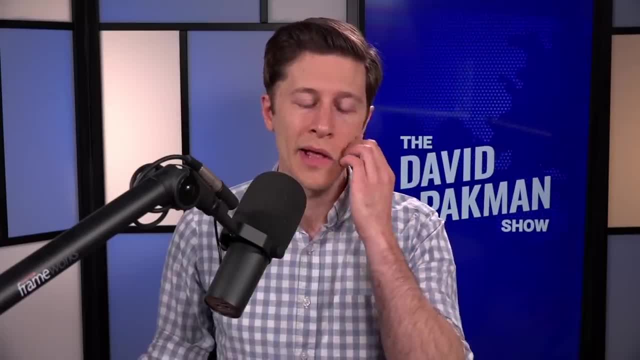 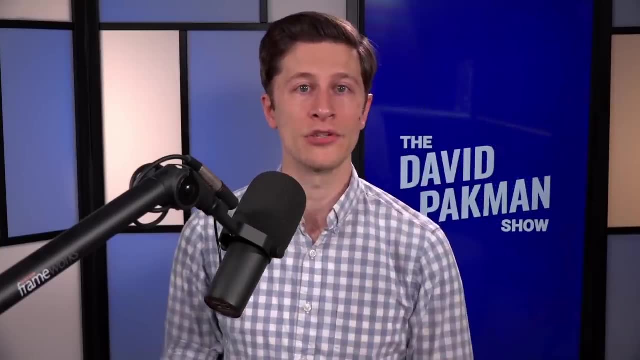 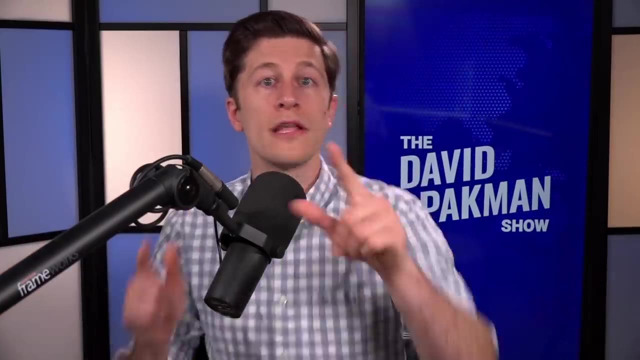 transparent political attack. There's no question about that. But the degree to which it's transparently bogus is only becoming more clear now, as we start to get this data, as we emerge from the pandemic, And they're not going to change their tune, But hopefully you now.